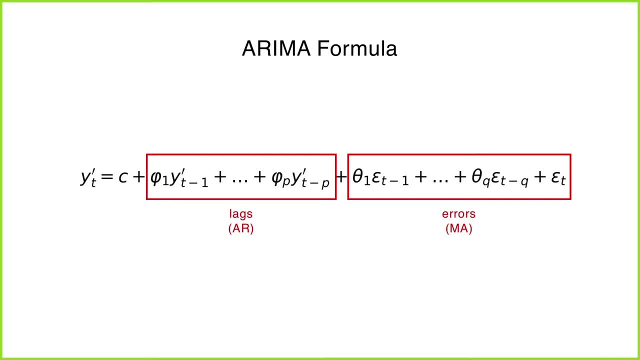 and the future values that are found in those past values. so, in short, arima models explain a time series based on its past values, basically its lags and and its lagged forecast errors. so an arima model is characterized by three terms and these are the: 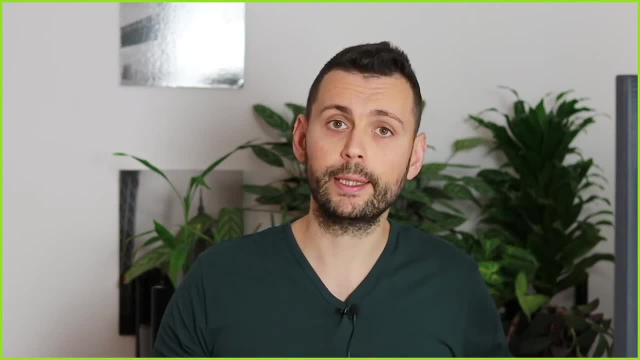 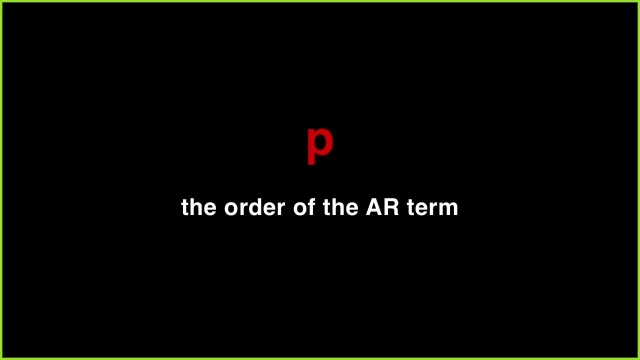 most important things that you need to know in order to be able to fit an arima model, and these are p, d and q. all right, so p refers to the order of the autoregressive term, d is the order of differencing, in order to make the time series stationary, and q is the order of the moving. 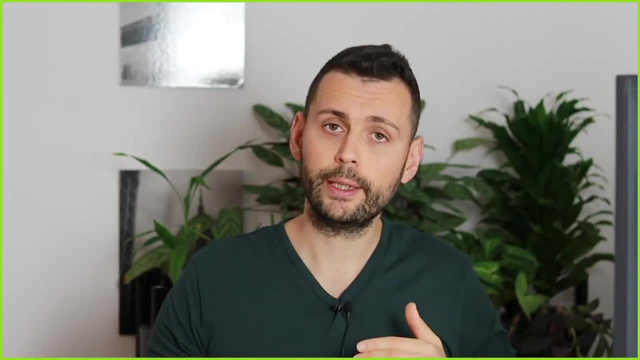 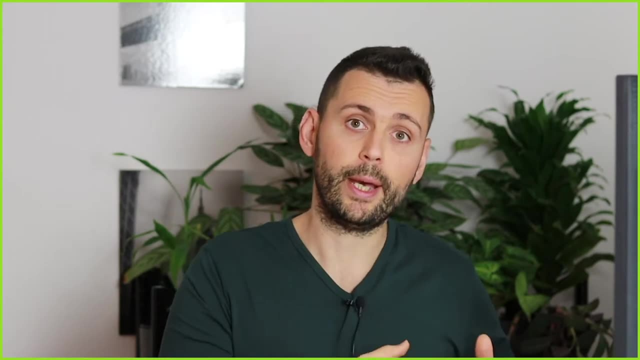 average of the moving average and q is the order of the moving average and q is the order of the moving average term. now we're going to go through all of these three and i'm going to explain how they are calculated and how you can actually get these values so that they are mapped perfectly to your 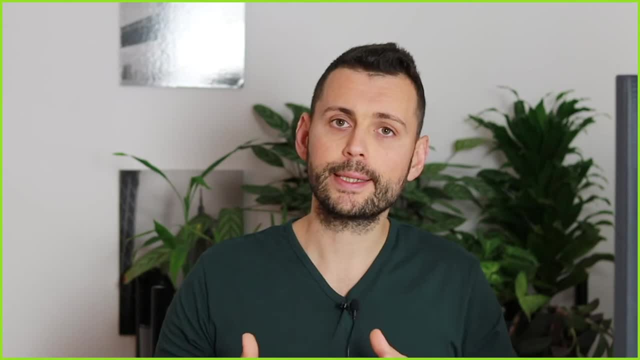 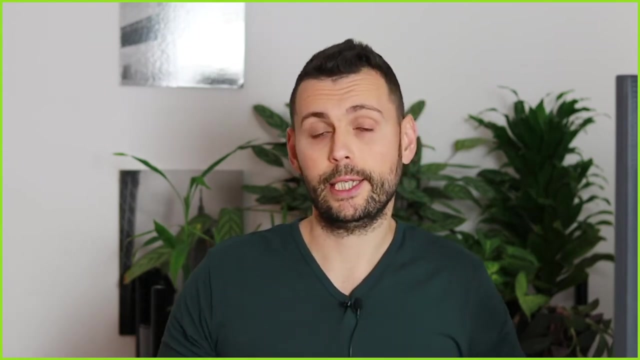 specific problem. but as we see from these terms, we realize that what we actually need to have in order to be able to fit an arima model is a stationary time series. okay, so the time series needs to be stationary. you might be wondering: what is stationarity? 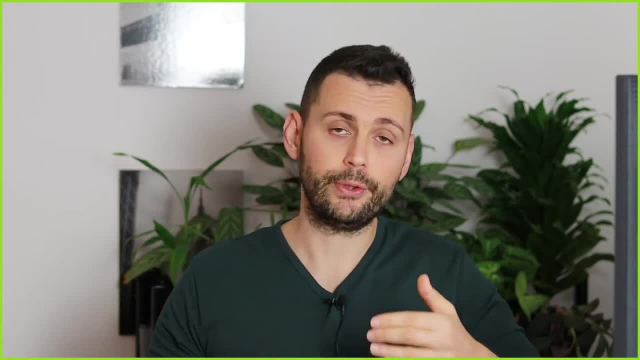 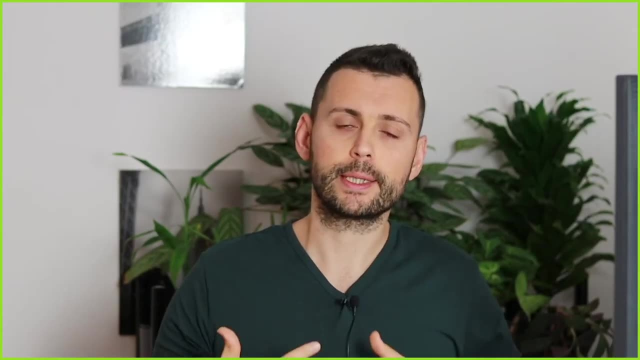 now stationarity refers to the fact that the price series in this case is mean reverting and, as we know, most price series aren't mean reverting because otherwise it would be super easy for us to be able to profit from, uh, from the stock market. because 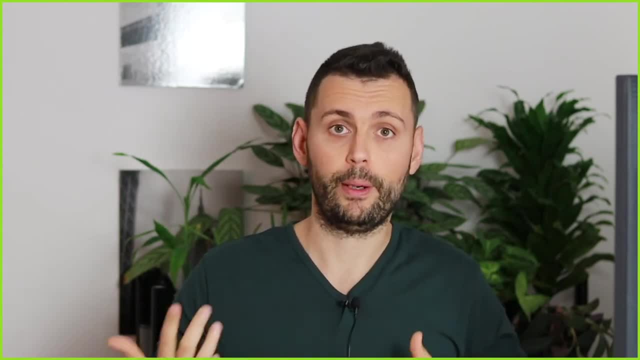 we would only buy low and sell high, or the opposite, okay, we would short high and then buy low. but we know that this is not the case, because prices don't mean revert you usually, and the ones that do are very rare. but what we do know is that the returns 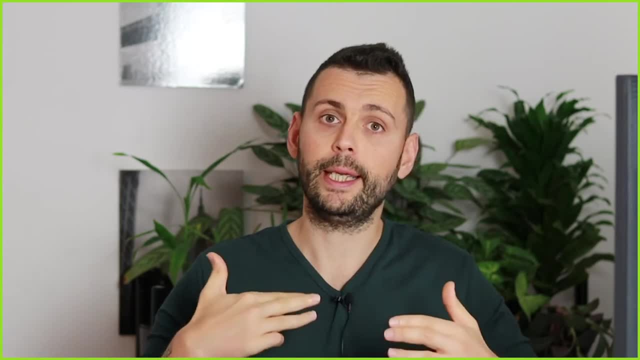 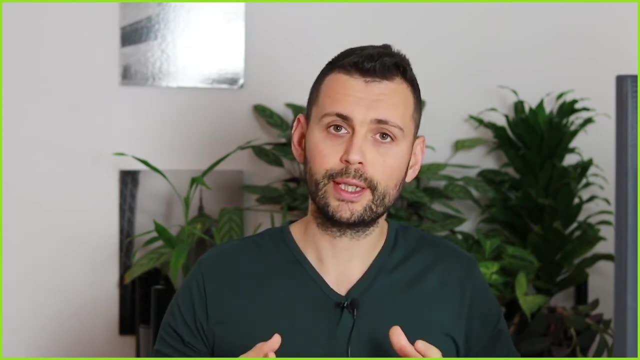 are more likely to mean revert because they are distributed randomly around a zero mean. so, coming back to the arima model, we know that now we need a stationary time series in order to be modeled by an arima model. but why is that? and the answer lies in the autoregressive term in the 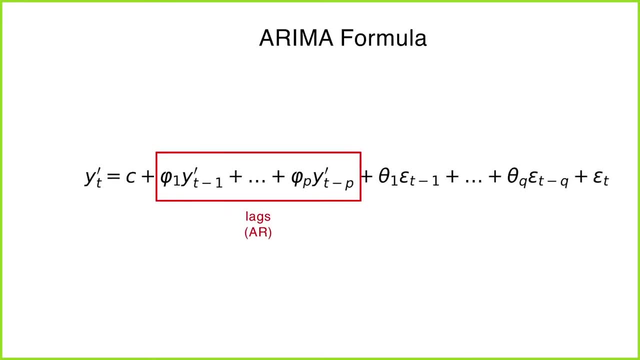 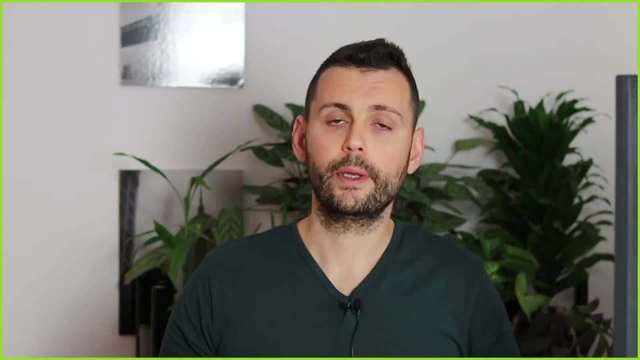 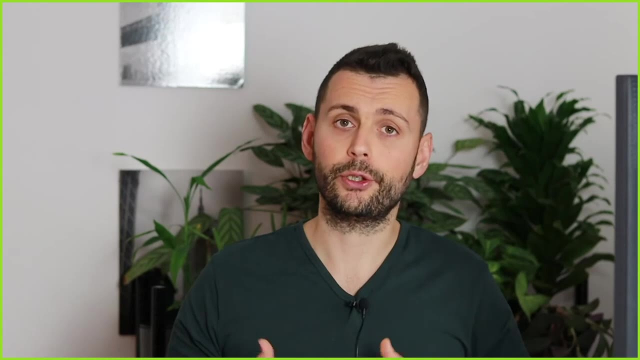 actual name because it's autoregressive. it means that the model is a linear regression that uses its own legs as predictors. now, linear regression, as we know, works best when the features, when the predictors, aren't dependent on each other, because if they are dependent, that means we will run into the problem. 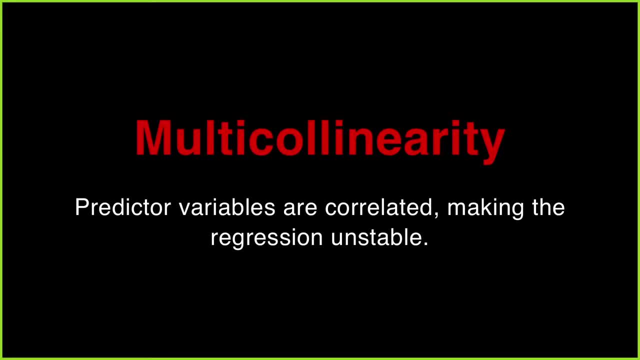 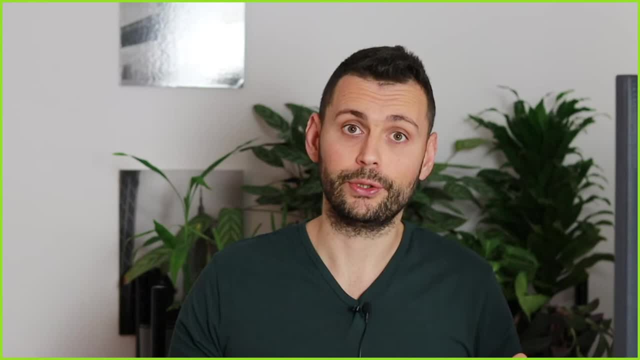 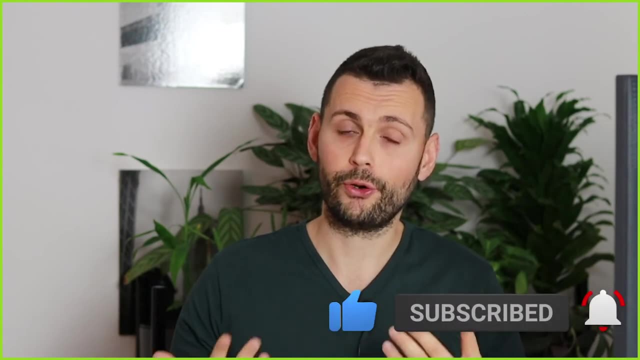 of multicollinearity. in that scenario, if these predictors are correlated, our linear regression will be unstable and it might not reach a result. so it's super important for our predictors, for our variables, to be independent from each other, to not be correlated, and therefore that's why we need 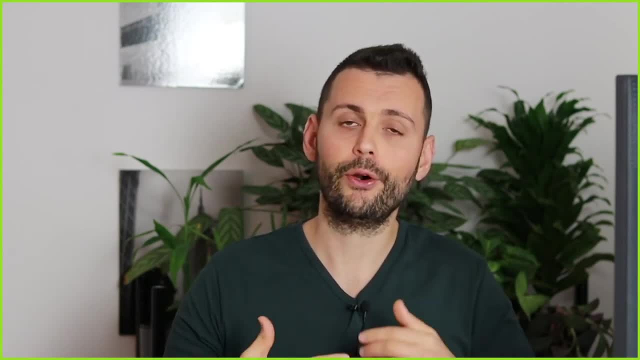 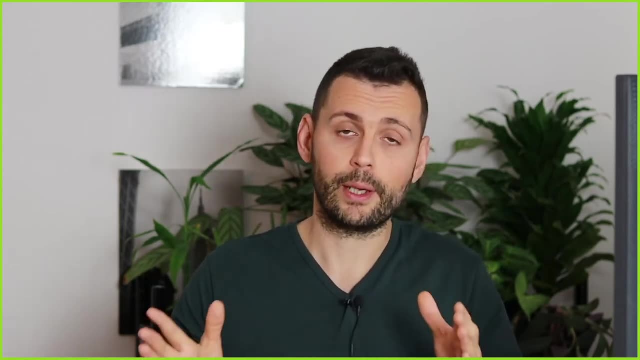 to make sure that our series is stationary or at least close to stationarity, because we might not be able to reach perfect stationarity and that's not necessarily a problem, but nevertheless, the whole point here is to get uh to a stationary time series if we can. but 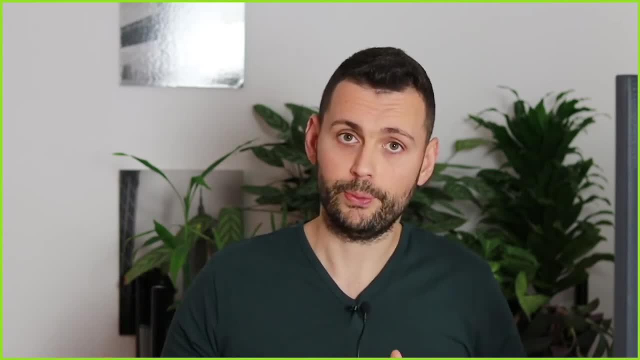 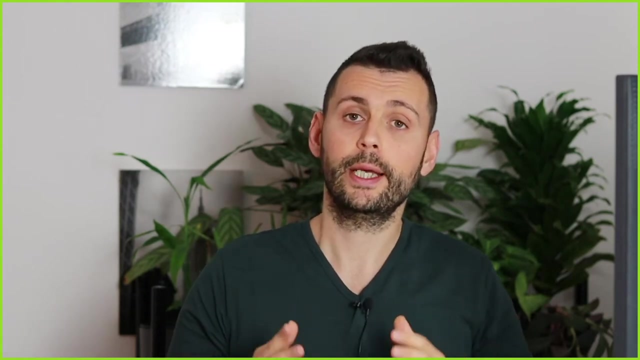 least to have a mildly stationary time series, to be able to model it with an arima model. now, as i said earlier, price series usually are non-stationary, but we can get stationarity if we get the returns, because those guys revert to the mean. that is exactly what differencing is. now let's go through. 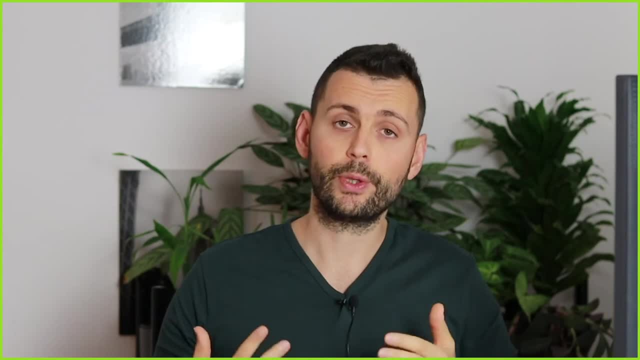 a practical example through this microsoft price series, so we can see exactly how everything works. and then we're going to explain all of the terms that are required by the arima model to be actually fitted to the data. okay, so let's go ahead. the first thing that we're going to do, 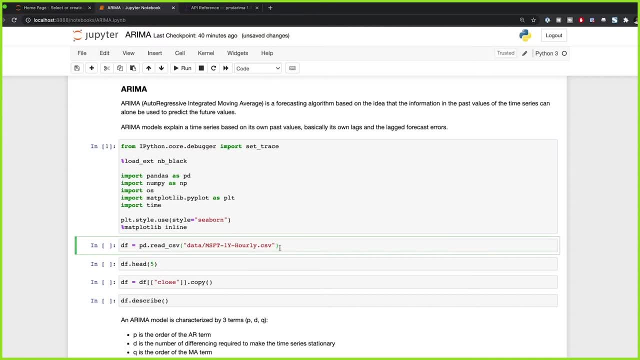 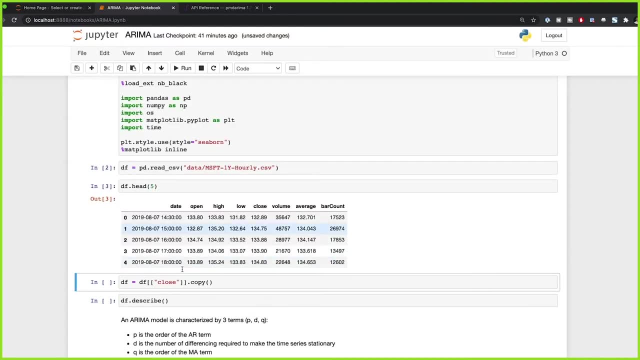 of course, is import the necessary libraries and we're going to read our microsoft hourly data. this is over one year. let's actually see the head and we can see. we have the open, high, low, close, volume average and bar count, but we're only going to be using the close. 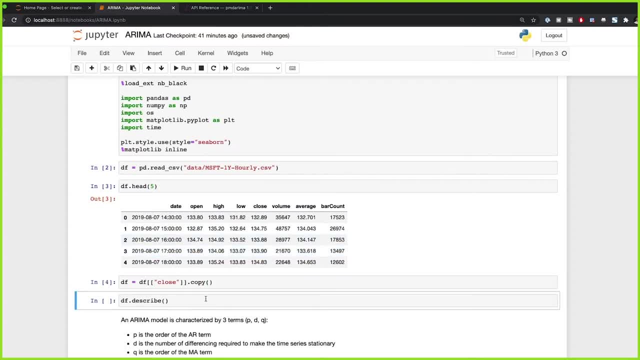 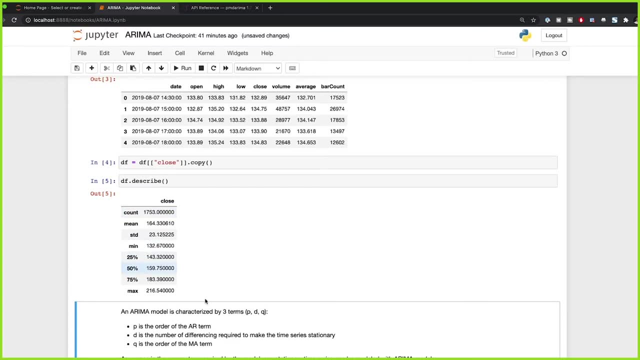 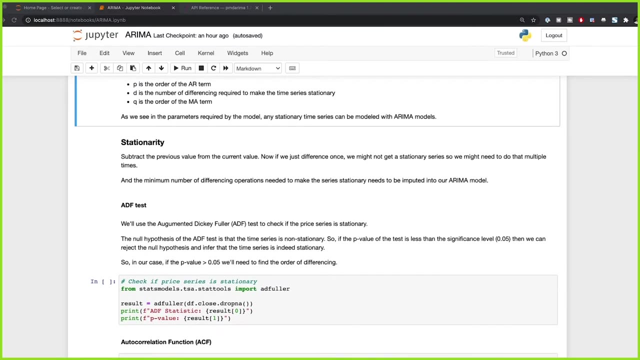 so let's just create a copy of this data frame with just a close feature, and if we describe it, we can see these stats. so now you might be wondering how can we find out whether a price series is stationary- and that is done through the augmented dickey fueler test and what the adf test does. it tries. 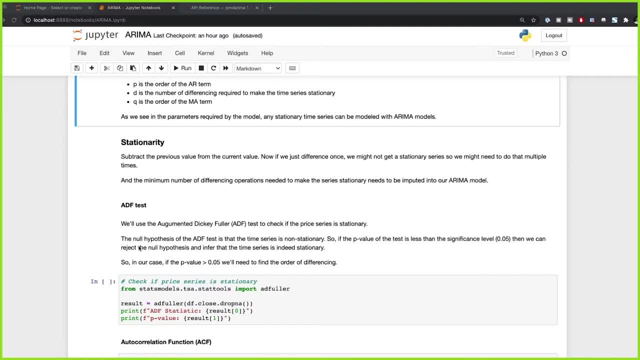 to prove the null hypothesis wrong, all right, and our null hypothesis is that the time series is non-stationary. so if we prove that the time series is not non-stationary, then there is a huge probability that it is stationary, and that is what the adf test does. so if the p value of the test is less than the significance value of 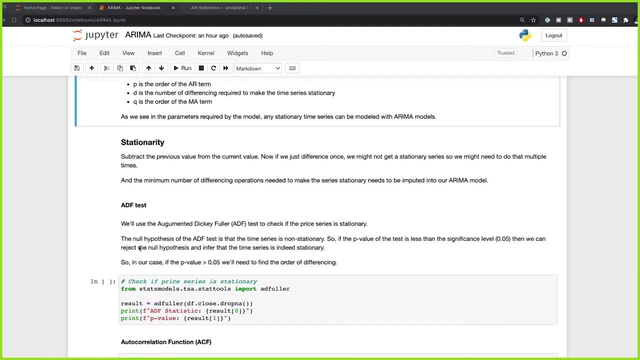 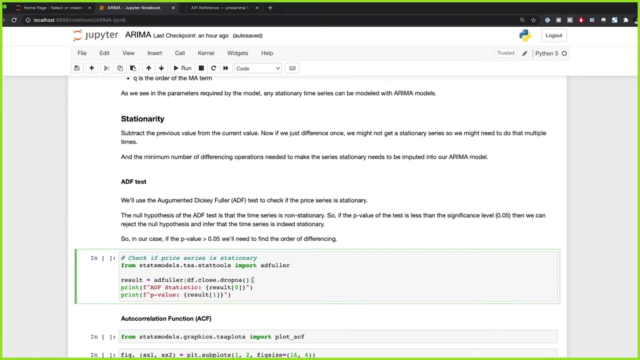 0.05, then we can reject the null hypothesis and infer that the time series might be missionary. so in our case, if the p value will be higher than 0.05, we'll actually need to find the order of differencing, and you're going to see that if we run this okay. so we're going to 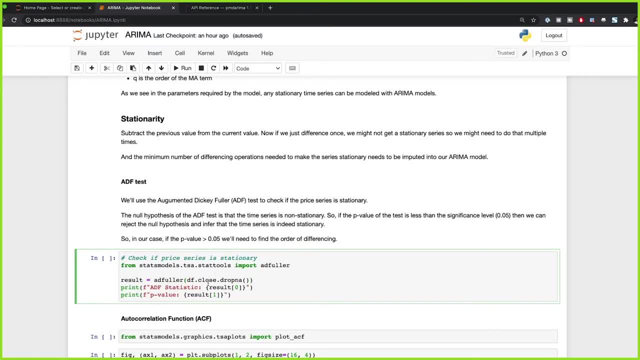 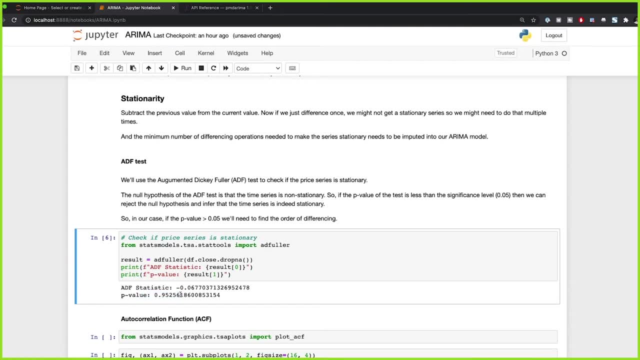 import ad filler from stats models and then we're going to apply it on the close prices. we can see that we get a p value of 0.95, so it's quite high, right? so it's clear that this price series is not stationary. now most prices are non-stationary because 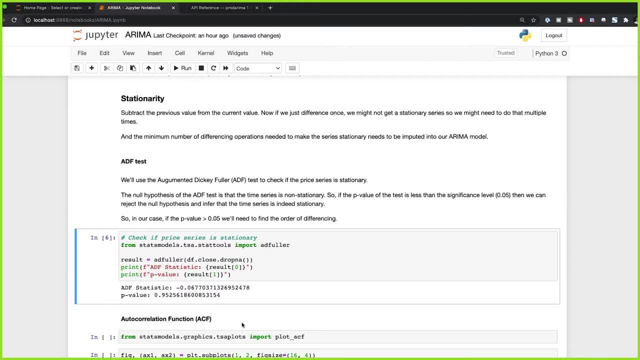 otherwise, as i was saying, we would all be super rich by just buying low and selling high. so in order to make these arima models work, we need to difference them. so in this case, we're going to have a p value of 0.95. so we're going to have a p value of 0.95. 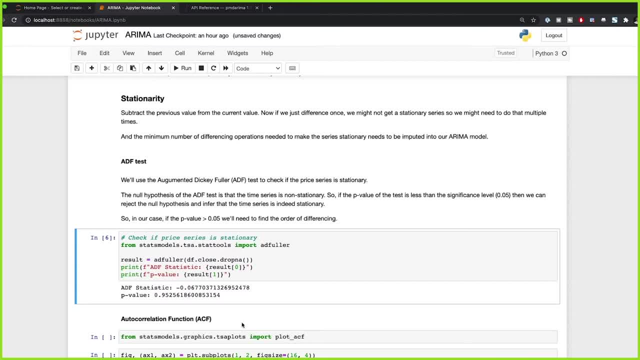 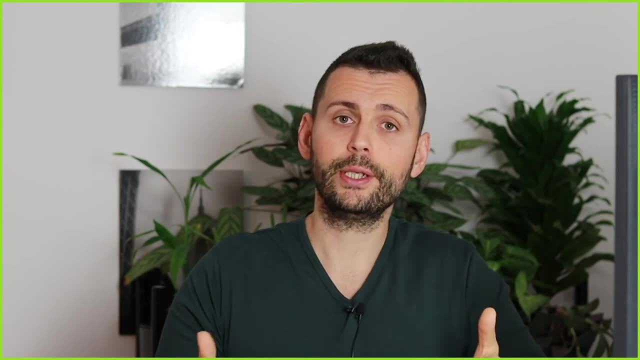 we will need to compute the returns, as they usually randomly distribute around a zero mean. we just simply need to subtract the previous value from the current value. now, if we just difference once, we might not get a stationary series. so even the returns, if we just difference once, won't be stationary, so we might need to difference multiple times. we will need to get 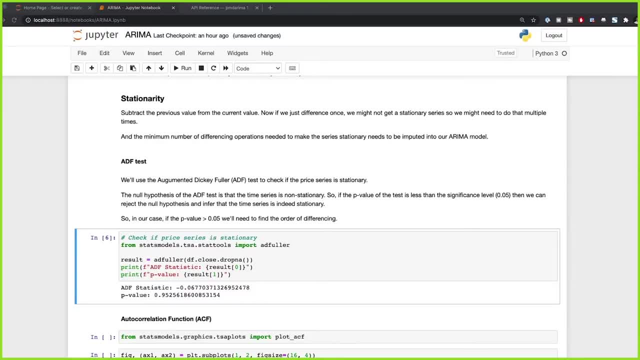 the returns of the returns and therefore we can have multiple orders of differencing. and that is the d term in our arima model and the minimum number of differencing operations that we need to make this actual time series stationary needs to be imputed in our model. so if the time series 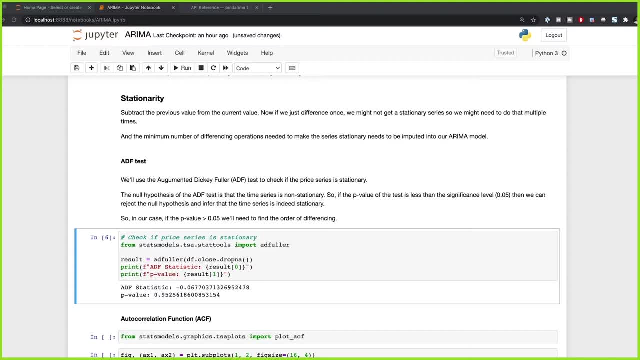 is already stationary, d is zero- but otherwise we will going to need to input the order of differencing that is suited for our time series and the way we can do this manually. to find the order of differencing, we can actually use the order of differencing that is suited for our time series. 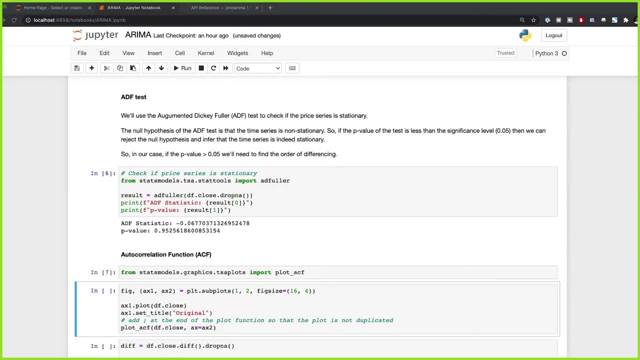 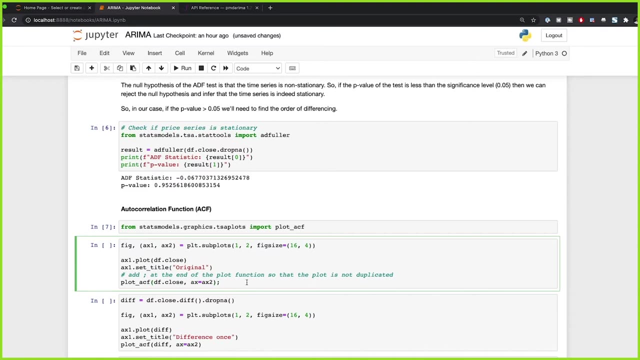 and we can use the acf plot from stats models and the acf plot tells us how many terms are required to remove any autocorrelation in the series. if we run this, we're going to first plot our close price and we just need to add. 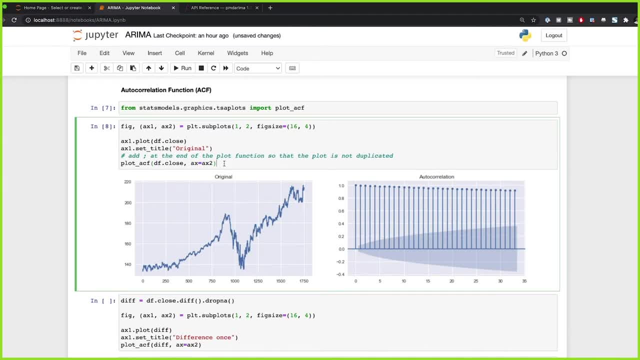 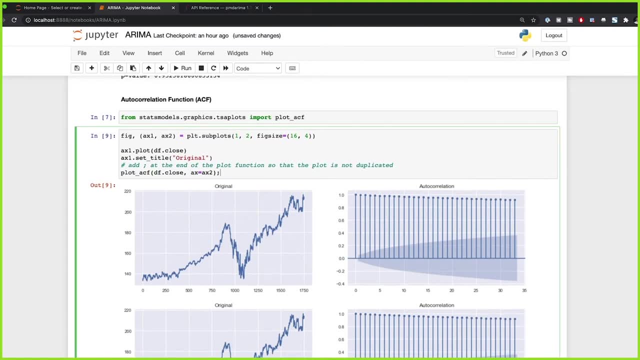 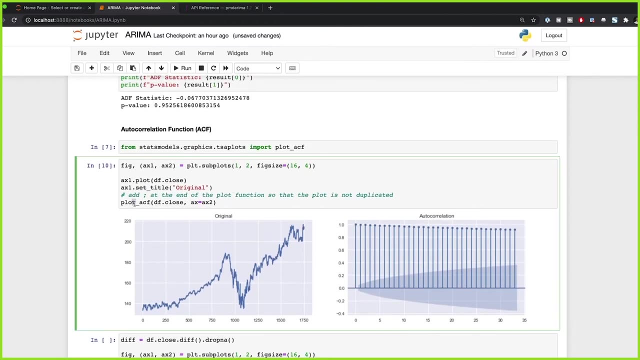 this so that it only plots it once, because if i would run it without that we would get two plots. so we just have to add this and run it again so we see we only plot it once. it's like an error in the plot ACF method so we can see our original price series and the autocorrelation. 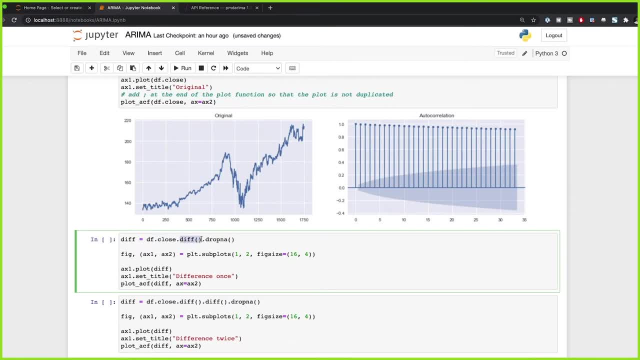 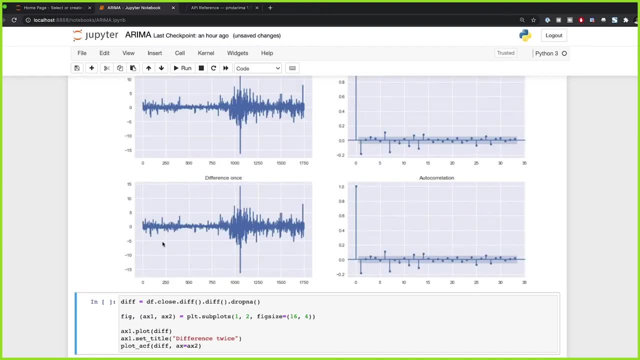 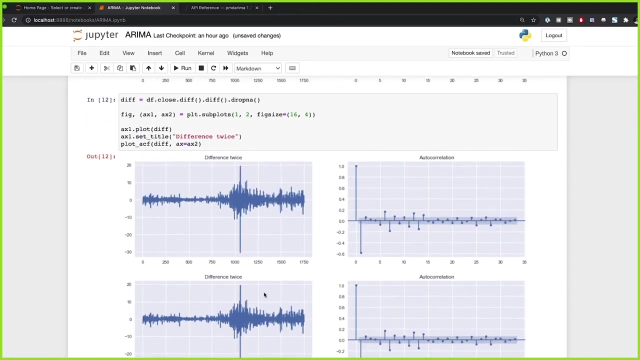 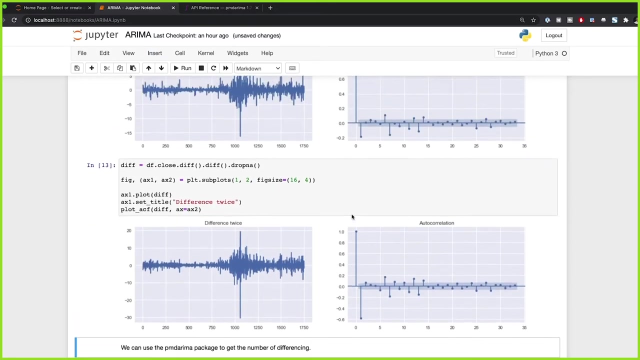 after we difference it once, we can see that we're getting the returns of the close price. we can see that now our returns they randomly distribute around the mean of zero and the autocorrelation plot looks like this: now, if we would difference them twice, let me just add this so we don't double this again: it's: 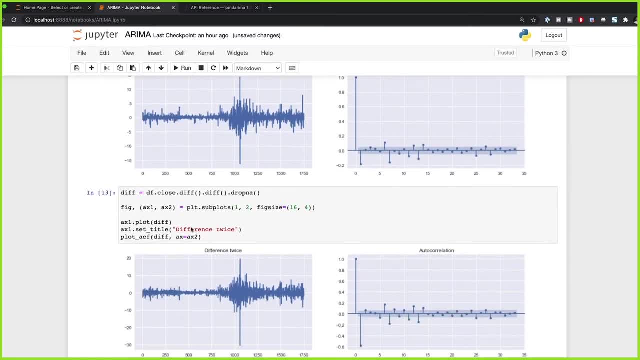 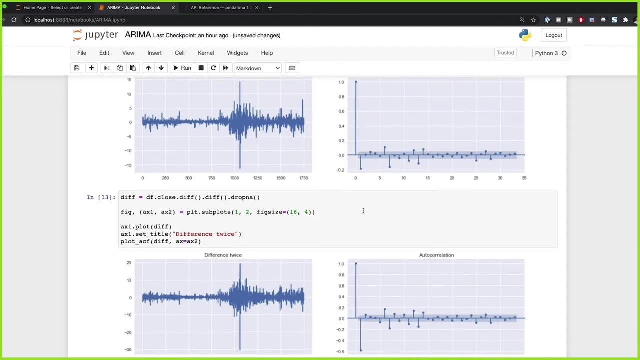 not much of a difference when we difference twice relative to once. okay, so our autocorrelation plot looks pretty similar. it's just that in the second differencing the lag goes into the far negative compared to the first order of differencing. so that may indicate that the series might have been over different. so therefore we're just 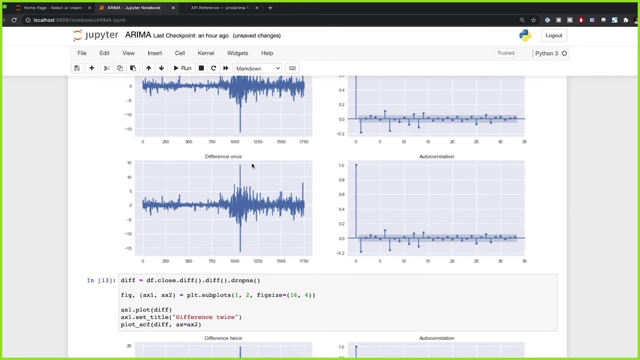 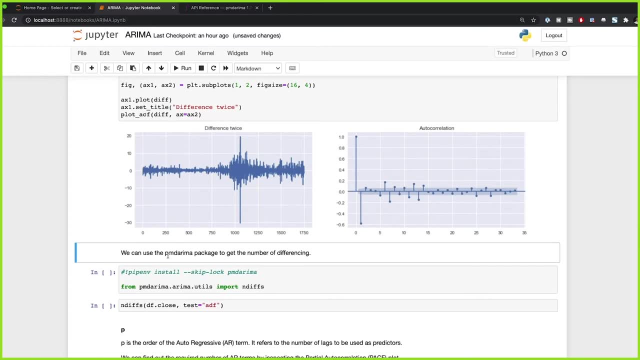 going to choose our order of differencing as one. of course, we can also use the PMD arima package to get the number of differencing, and this is a very, very helpful package. all we have to do, we have to install it. it's simple. we. 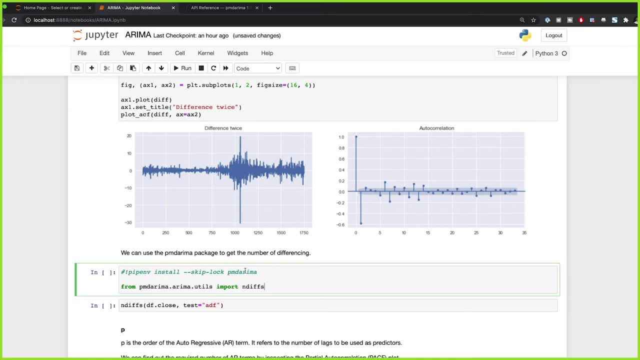 can install it with pipen install and PMD arima, or we can install directly with pip install, PMD arima, and then we import and ifs. and it's very simple. we just get the number of differencing for the close prices and we're going to run the ADF test. 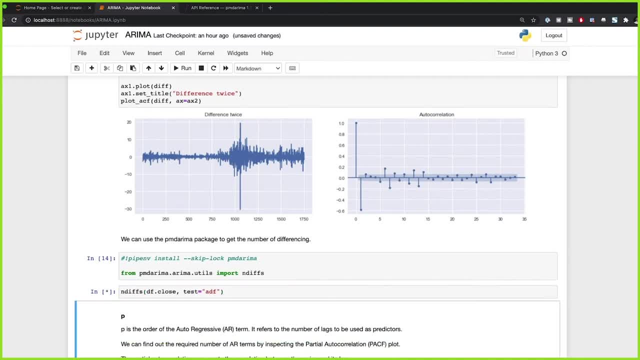 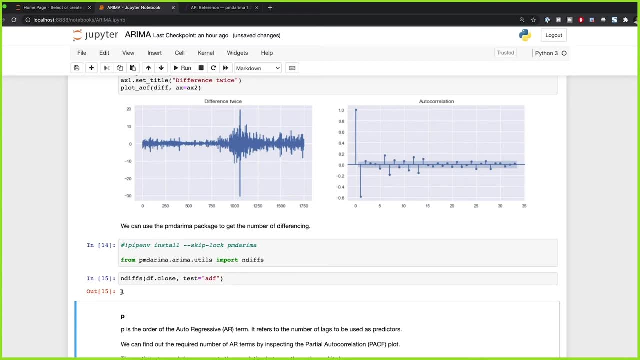 exactly how we run it manually above, and if we run this, we will get one, which is the number of differencing that is required to make this series stationary, and we got the same result here. so we can see that the number of differencing that is required to make this series stationary, and we got the 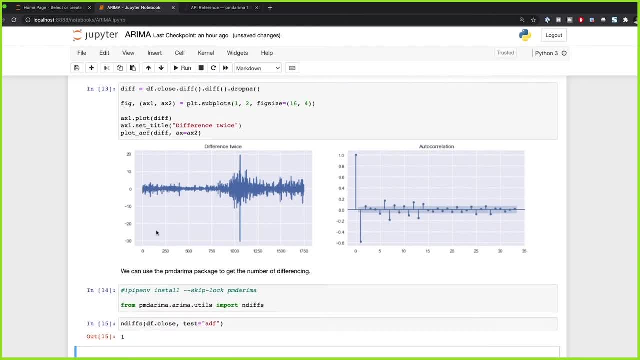 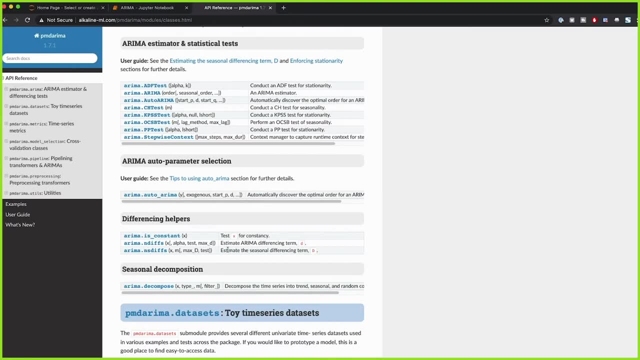 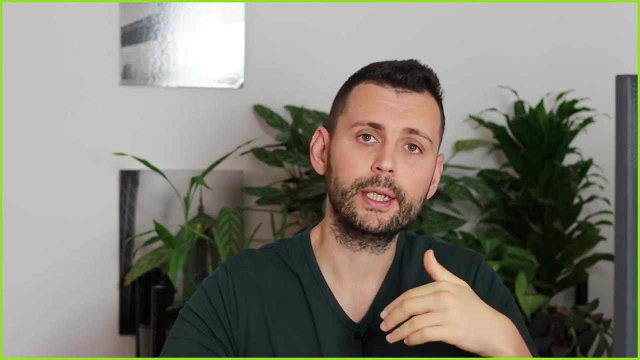 same result by analyzing the ACF plots. if we look at the API reference for PMD arima, we can see that ndiffs estimate the arima differencing term. this is super helpful for you guys to use in in your own application so that you don't have 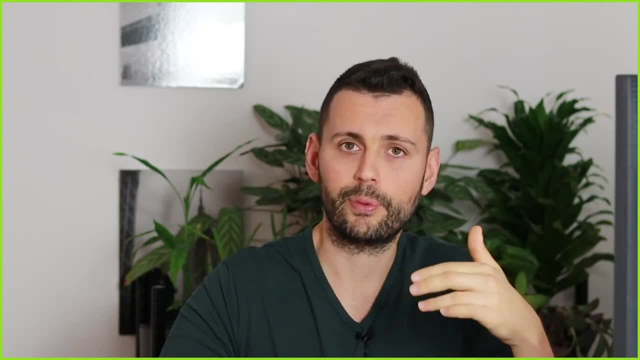 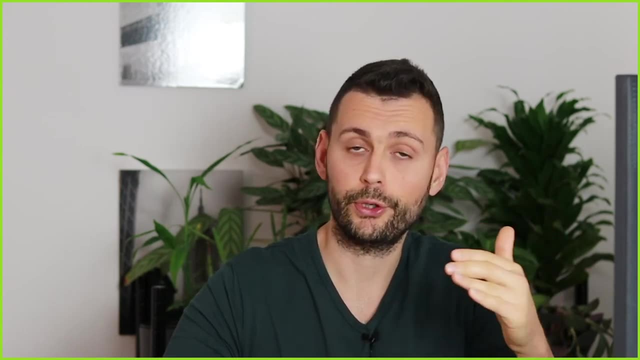 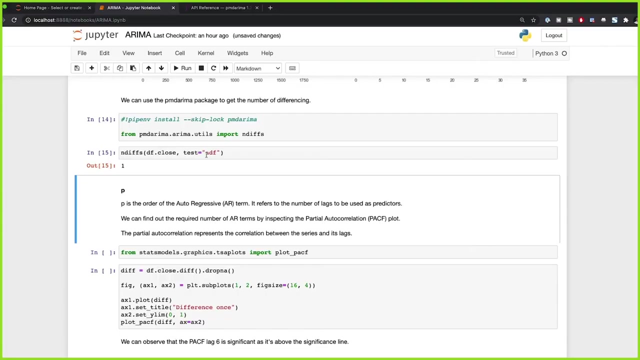 to do this manually and look at plots and decide manually if one or two or whatever order of differencing is appropriate for your problem. so you can use ndiffs just to get the order of differencing. this saves you a whole lot of time. let's go ahead and talk about the other terms in our arima model and P. 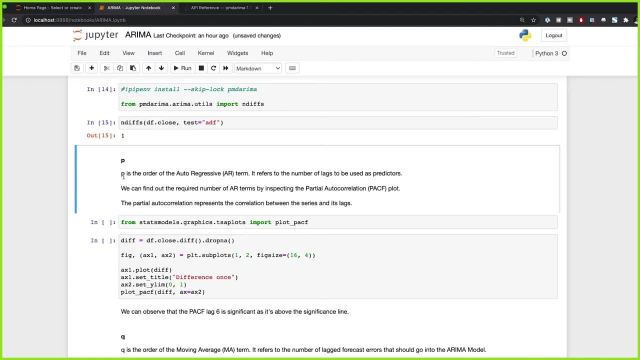 P is the order of the autoregressive term. okay, so the AR part of the arima model. it refers to the number of lags to be used as predictors. now we can find a number of required AR terms if we inspect the partial autocorrelation plot. 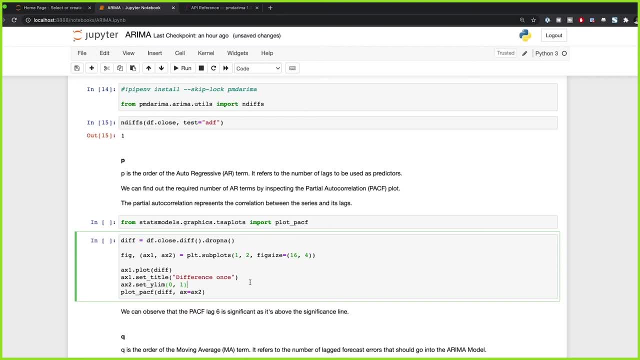 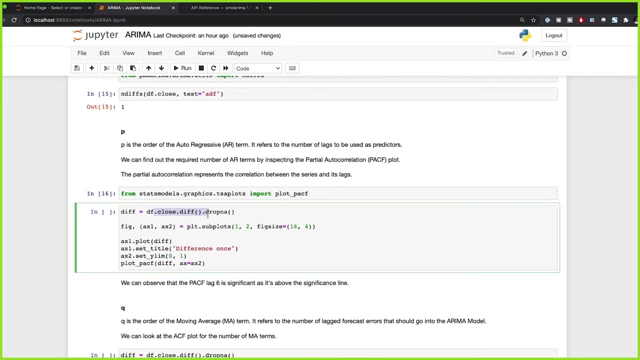 not the autocorrelation plot but the partial autocorrelation plot. so the partial autocorrelation plot represents the correlation between the series and its lags. so if we import this and we get, of course we're just going to get the first order of differencing, because that's the one that we chose for our 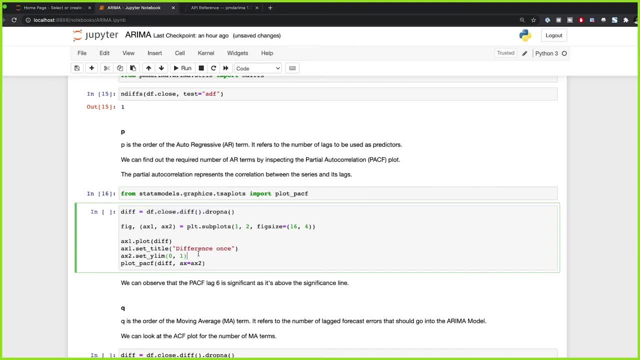 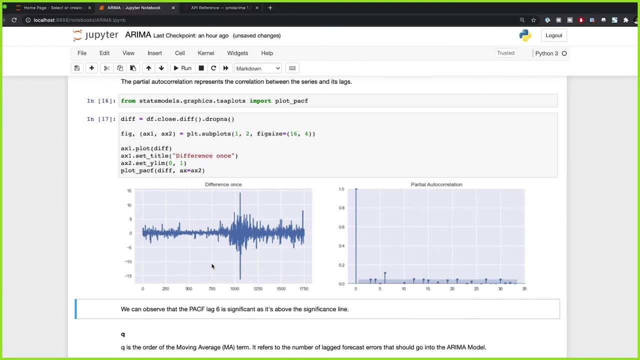 problem. if we run this- and of course we have to add this at the end- we can see that the partial autocorrelation plot looks like this: what we can observe here is that the partial autocorrelation plot- lag number six stands out- is well above the significance line. so even three and four. 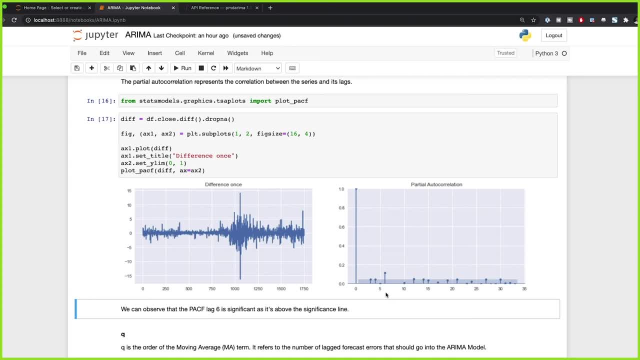 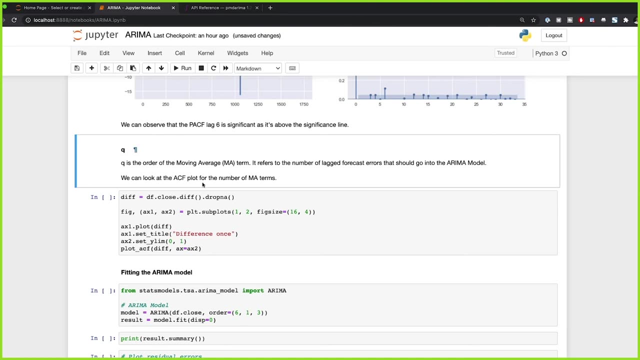 are a little bit above the significance line, so we could use three, four or six as our P term, but for this example I'm going to use six. now the Q term is the order of the moving average term, so it refers to the number of lagged forecast errors that should go in the arima model. so this: 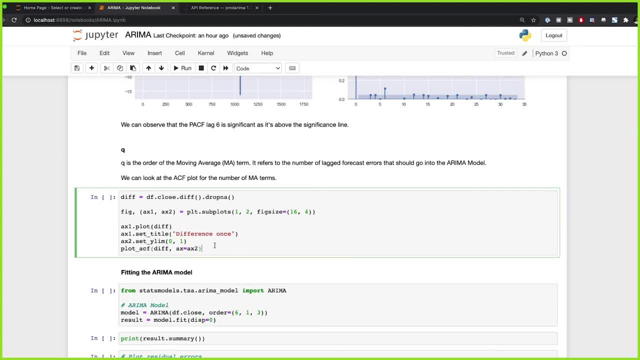 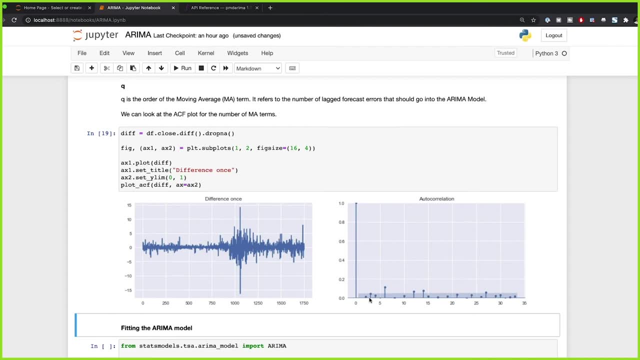 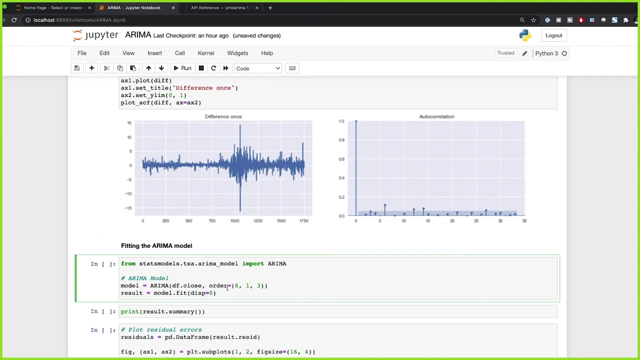 refers to the MA part of the model. so here we can plot the ACF plot for this specific term and here we can see that the forecast error three may be suitable for this model. okay, so we're going to choose three as our Q term. now that we have these three terms, so we have our PD and Q term. we 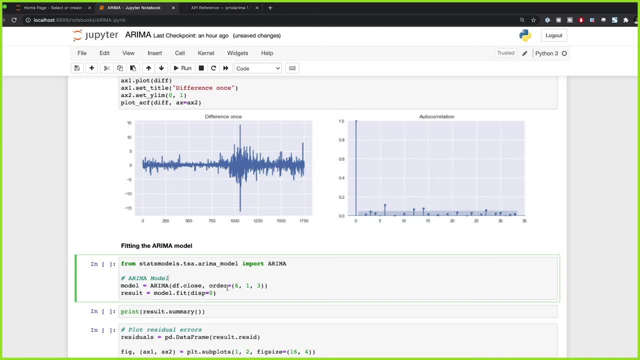 have P set to six, we have D set to one and we have Q set to three. now, of course, the queue, as you saw previously. we might even choose it to be zero, but for this example, we're just going to choose three, just because we can see that the 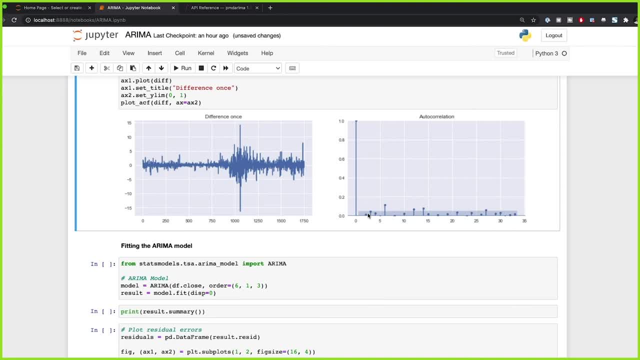 forecast error three is a little bit above the significance of this model. we're going to add our forecast error four times this time, so we can see here that the progress text should be rather over than the arpeggiated Pastor uncheck significance line. so we're going to choose three just for this purpose. so all we need to do is 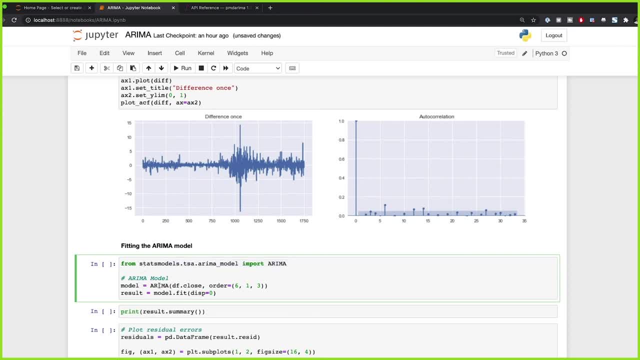 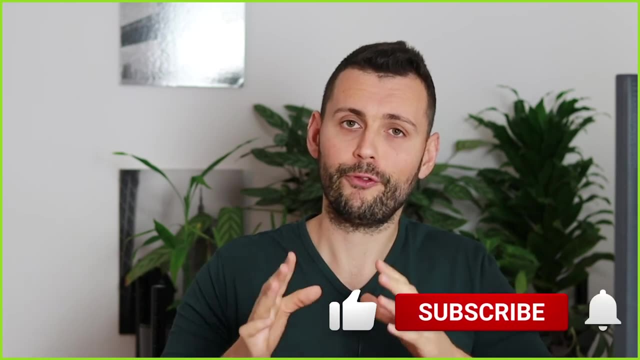 import arima from stats models and then we just have to pass in the series and then specify the order, so 6, 1, 3, and all we need to do then is to fit the model. but before i fit this model, i just want to thank you guys for subscribing to our channel and for liking our videos, because we 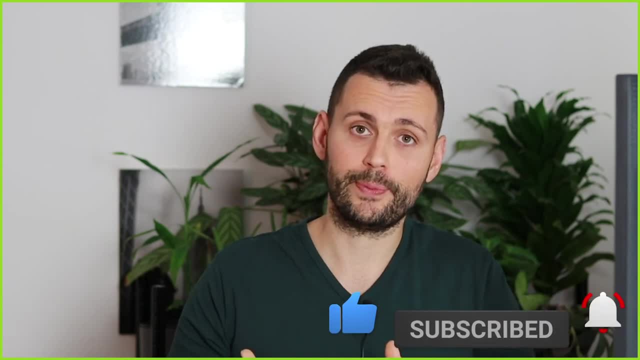 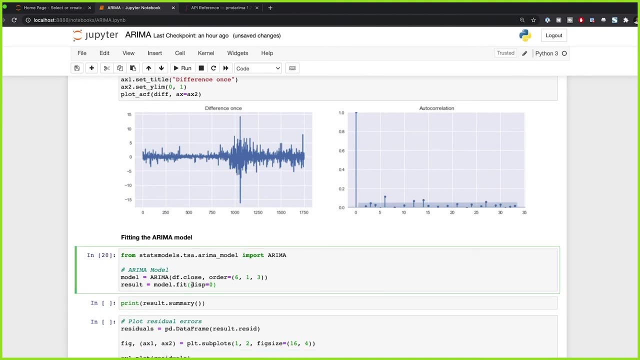 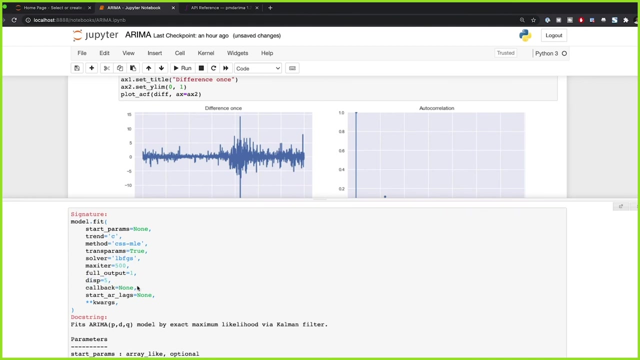 really want to help you guys grow in the data science and machine learning space, all right, so let's go ahead and fit this model. if we check the, let me run this. but now, if we check our fit method to see what it takes into account as arguments, we can see disp, just so that you. 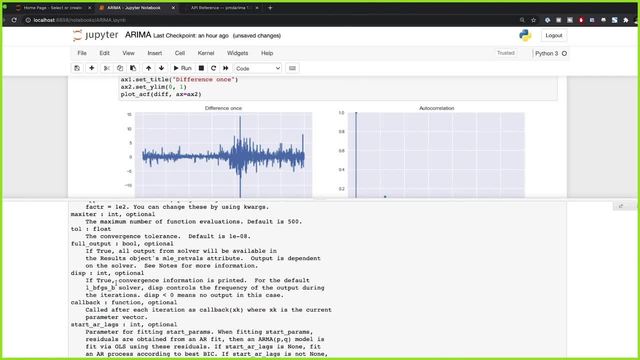 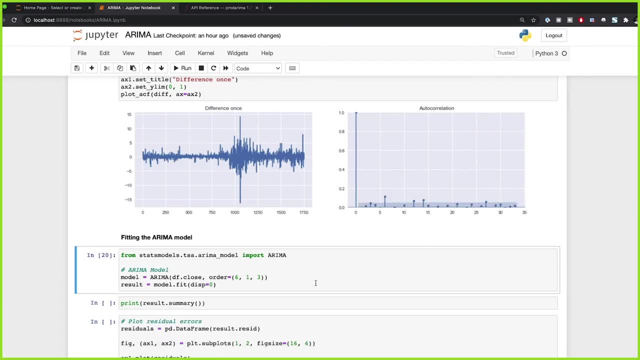 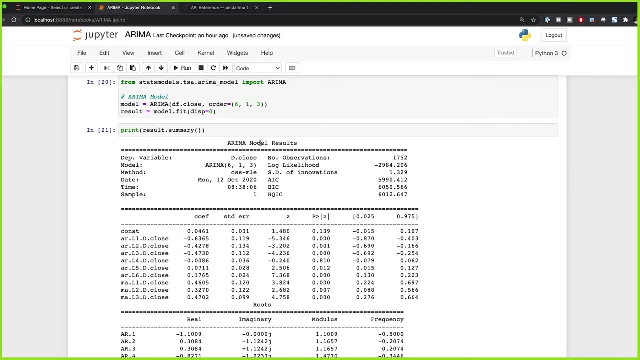 understand why i set this to zero. basically, converges, information is printed. i'm going to set it to zero so that it's false. let's see the result summary. and there you go. these are the arima model results. we can see that our ar terms: we have six ar terms and three ma.